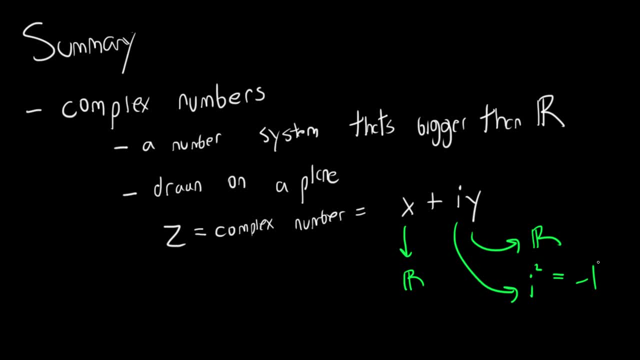 going to have the property that if I were to be squared it's going to be equal to negative one. That's going to be the special property that you have And to go about doing you know, multiplications and additions with these things. I'm not going to show you guys reviews of that. 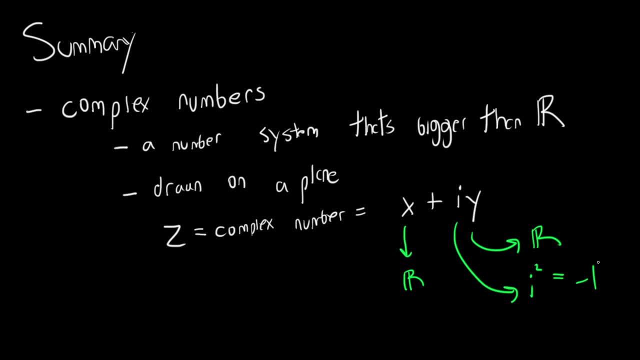 You're essentially going to just multiply them normally, using I as if it's its own variable. just leave I as its own And then every time you see I squared, you just simply replace it with I, that with negative one. That's essentially the trick to this. You're going to encounter that. 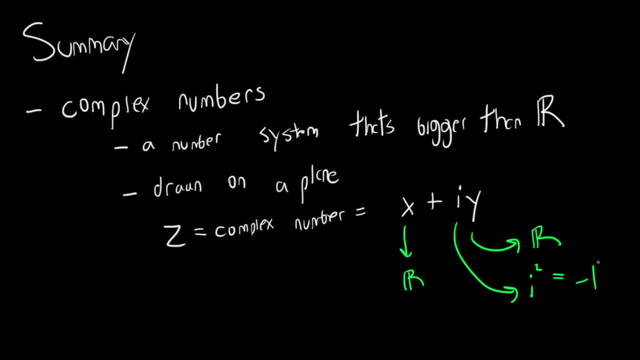 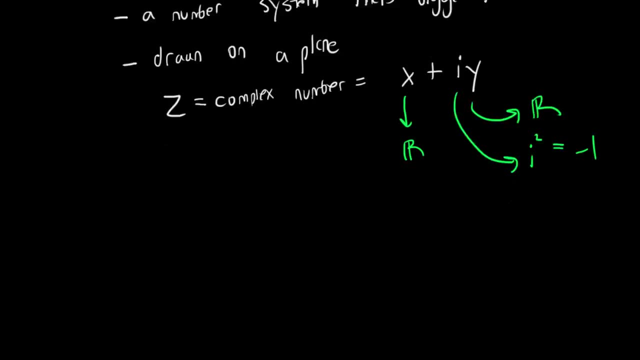 when you're dealing with multiplication and not with addition, obviously, because you're only going to have i's and no i squares. to begin with, We were introduced to the modulus. I might not have called it that, but we were introduced to the modulus- So the modulus of complex numbers. 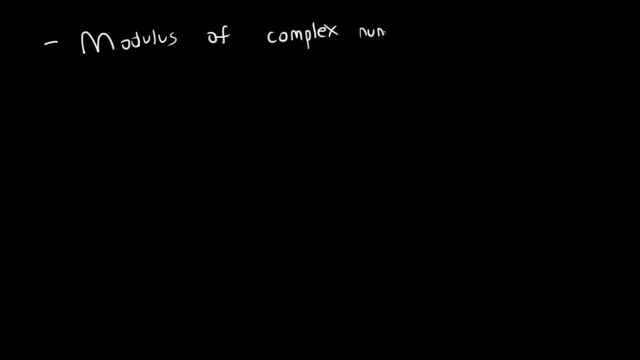 is z with these little bars around it. right, This will be the distance between zero and z and obviously with z having the coordinates x, y and z. I'm going to go ahead and give that a little draw over here. Say: we had our x, we had our y. 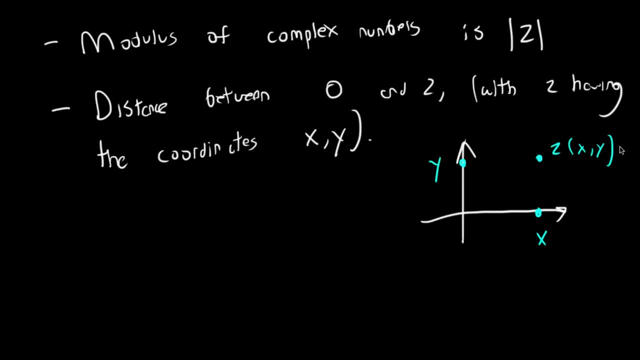 and we had our z, which obviously had the coordinates x, y, And we had: what color have we not used? Let's go with a nice orange? This here would be z. So this is the distance from your zero origin over here to the point z. 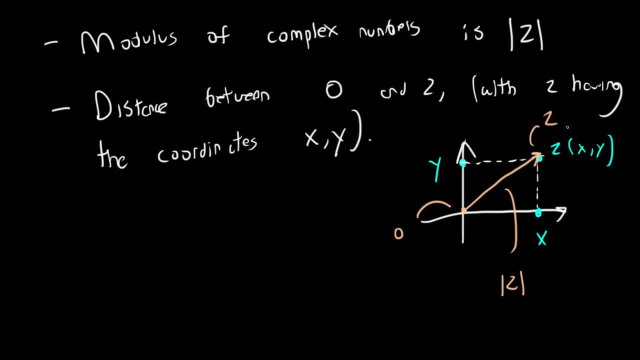 That's what it would be, What the modulus is going to be, And this would have the distance. So we can say would have the distance zero if it were on the real number axes, which remember this was this one down here, The x-axis, if you will. 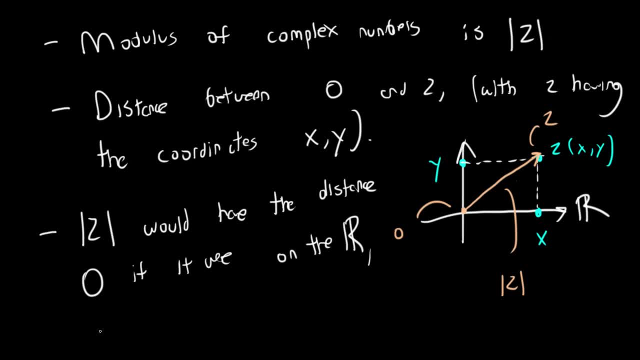 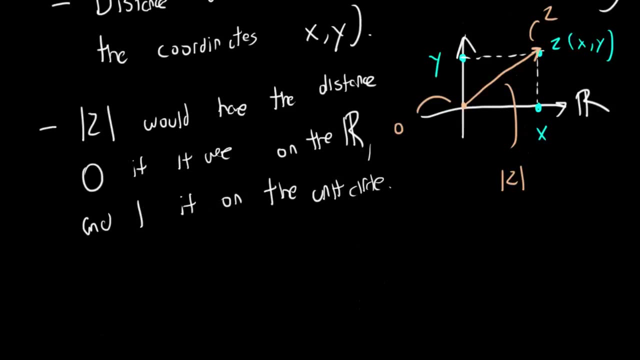 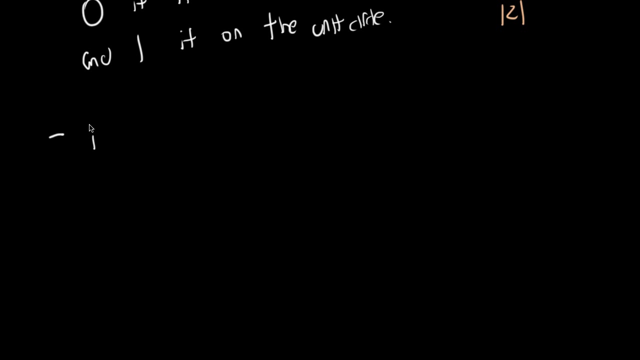 was for the real numbers And one if. on the unit circle We saw how we multiply by i and how that affects the plane, So we were introduced to. that was the problem. Sorry about that. That was the problem. we looked at when we would have i to the power of k, what that would change. 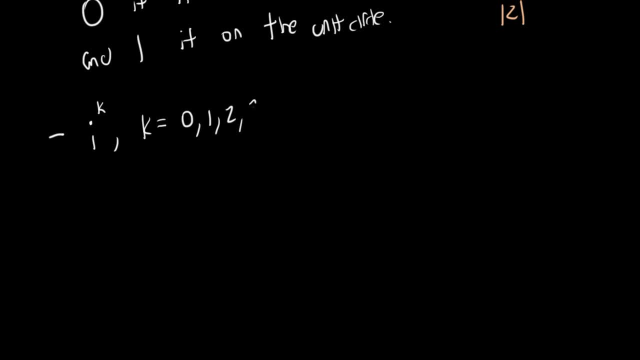 for k. I'll include the zero here. I didn't initially include it, but I showed you how to do it in that video. So how we would do it if k were to just be increasing like this And essentially we were to go ahead and we went and we graphed this out right. 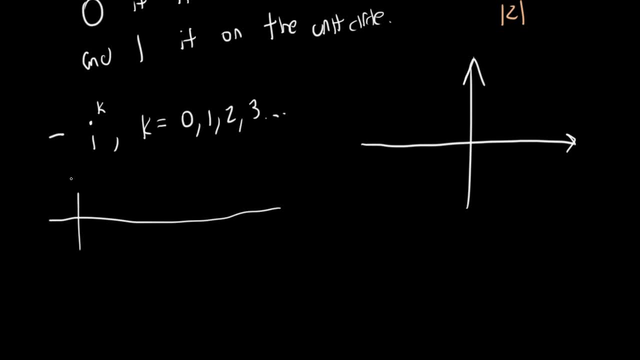 Because we would make a little table over here. So this would be our values of k, This is our values of i to the k, And whenever we're dealing with something like this, we want to find a pattern right And we saw that this was four periodic, which means every four values, you would have a repeat. 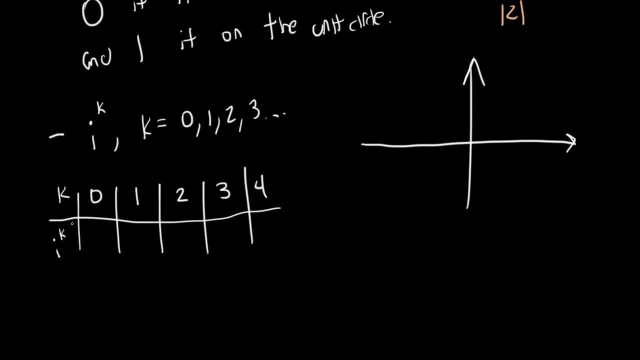 So I'll show you five values just to see that repeat. So what would happen if we have i raised to the zero? Right, If we have i raised to the zero, we know that anything raised to the zero is going to be one. 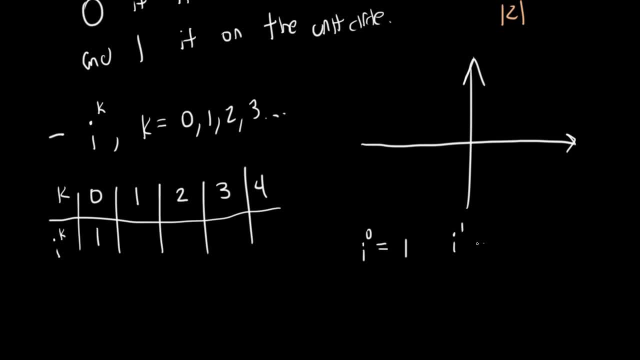 So we'd have a one over here. Then, if we had i raised to the one, we know anything raised to the one is going to be that value itself, So it's going to stay i. Then we had i raised to the two And we know that our special property, the one that we saw up here, 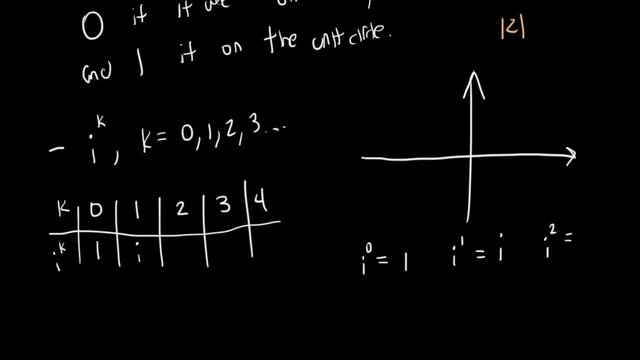 the special property that we have is that whenever you have i squared, you're going to have negative one, So we'd have a negative one here And then, when we got to the three, that's where things get a little bit tricky, Because you don't really see, you know how you'd go about solving this. 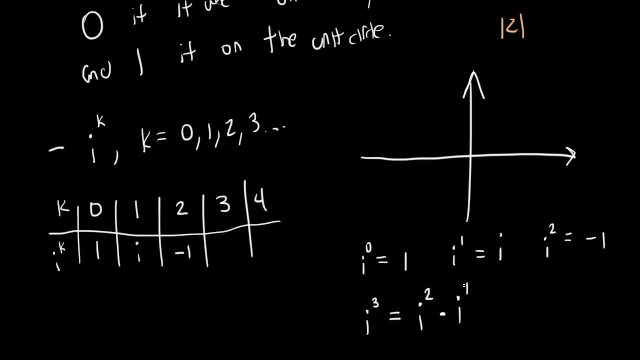 But essentially, when you can just go ahead and split these up if you wanted to, right. So if you have i squared multiplied by i, just to the one, that would mean using this property over here And this property, we would get negative one i, and that would just be negative i. 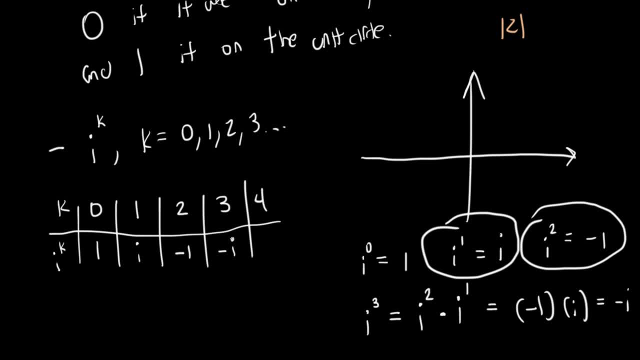 So we'd have a negative i over here And then dealing with the four right. the last one is to see that it actually does repeat. We start to split this up into i squared by i squared, which is going to be negative one. 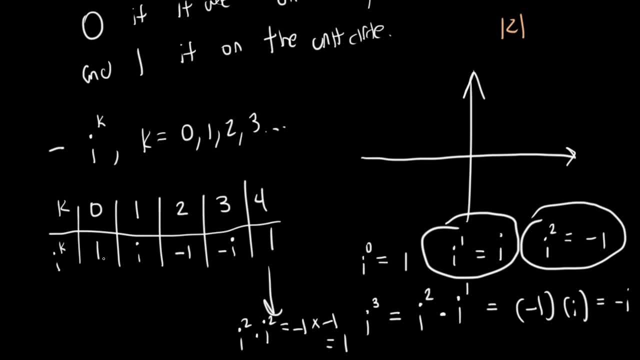 negative, one times negative, one, which is going to be one, and we see that we have the repeat of that over here. so we would we're able to go ahead and we were able to put that on this over here and remember this is still going to be representing r, so we'd have one over here and we'd have negative. 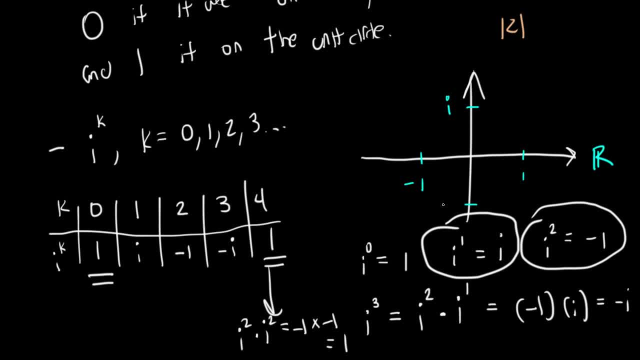 one over here, we'd have positive i over here and we would have negative i down here and essentially, every time you multiply by i, you are doing a rotation of 90 degrees, if you will around this circle. so that's one thing. we saw how multiplying by i were to affect something it's going to. 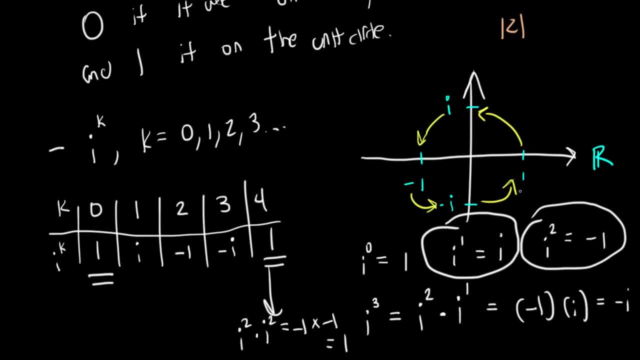 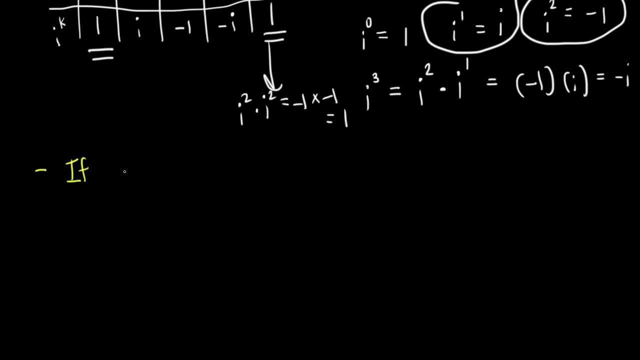 multiply it, it's going to make it turn around like this. uh then, therefore, right, if you were to multiply by i four times. so if you multiplied. so, multiply by i four times is i times i times i times i, which is i, to the power four, you will have no change. 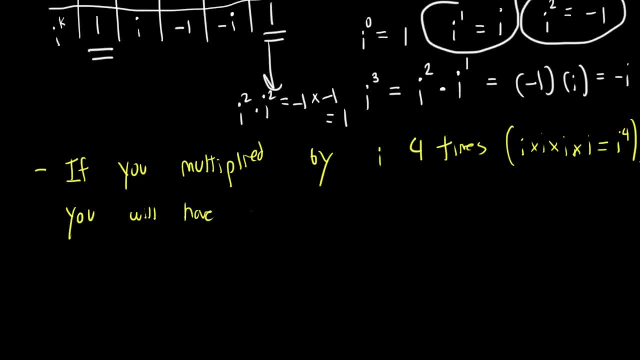 due to the four periodic right. every time you do four rotations it repeats itself. so you can multiply by i four times without having any consequences. you're going to wind up in the exact same spot that you started off. what were some other things that you were able to do that you were able to do that you were able to? 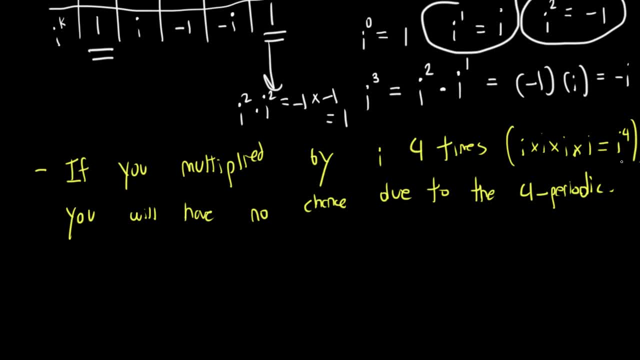 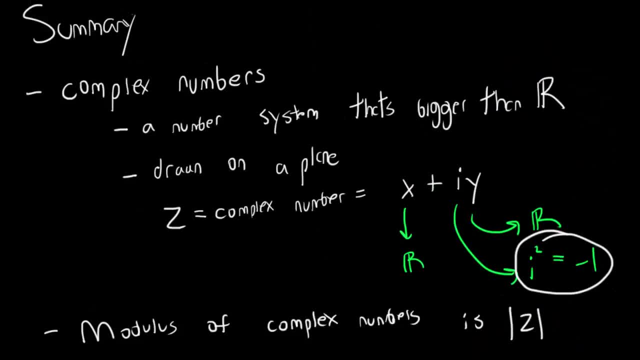 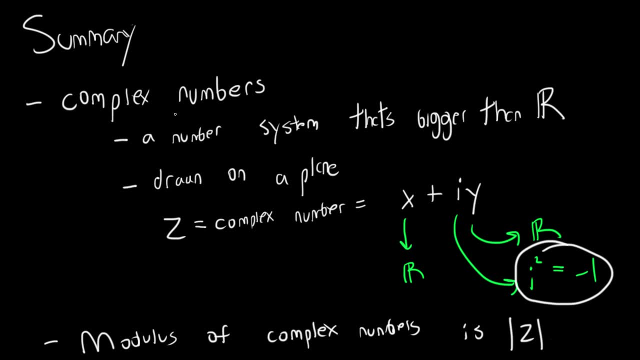 important in terms of just right now. I'll probably make a bigger video on those things, so don't worry about that. so that's what we saw right now and the rest is what we had from earlier videos. so we started up here with summary. so thank you very much for watching, and this was just a small 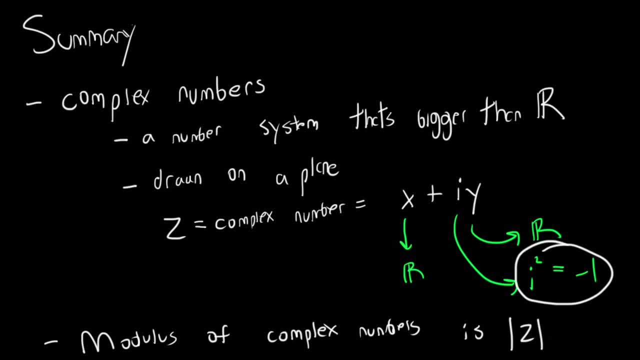 summary, I'll try to include a few of these every few videos to make sure we are all on the same path. so you know nothing new was covered in this video. if you have any questions, leave them below any questions on any of this material that we've seen or anything you'd like me to cover later on. 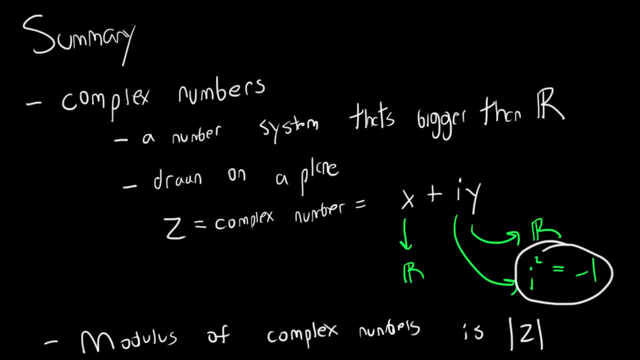 the series. leave below. I'll either answer you or make you a personalized video just for your question and I'll link it to you. and if any of my videos have helped you out, please subscribe. it means a lot and I will see you guys in a later video. bye.